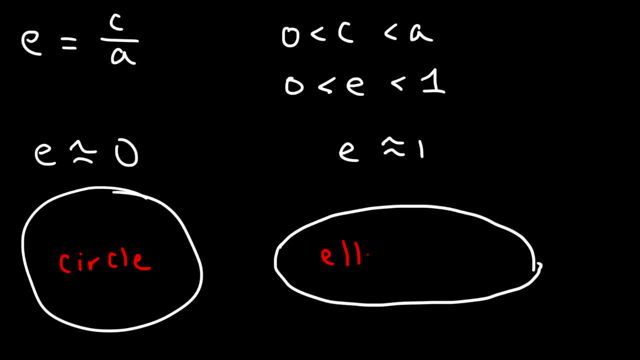 It's going to be elongated. And so E describes the shape of an ellipse. That's the purpose of an ellipse. That's the purpose of the eccentricity. 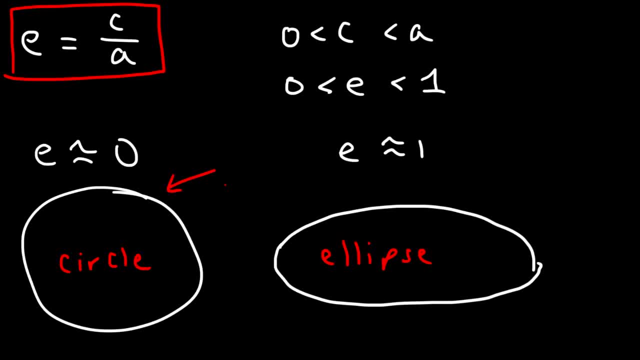 It tells you if the ellipse appears to be circular, or does it have an oval shape. Let's work on some examples. 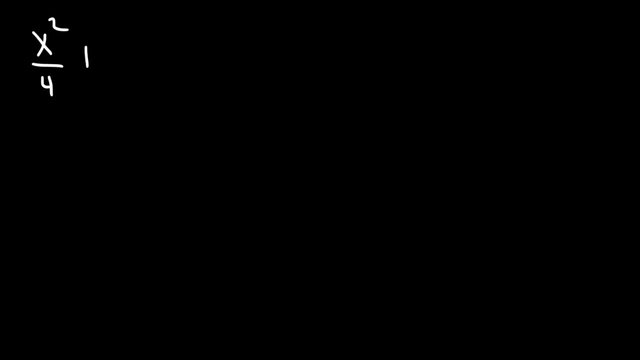 So let's say if we have this equation, X squared over 4 plus Y squared over 4 is equal to 1. Determine the eccentricity of this particular equation and go ahead and graph it. So the center is 0, 0. 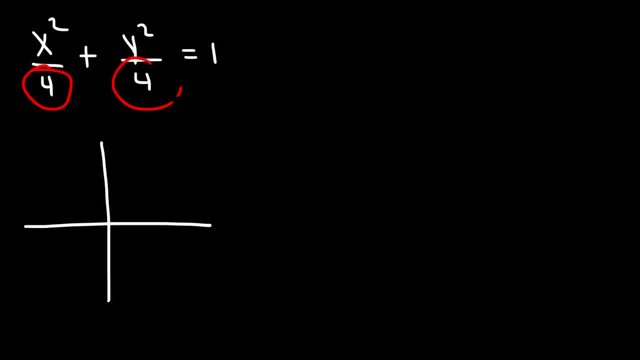 So the left is equal to 1. And let's call this A squared, this is going to be B squared. So this equation is in the form X squared over A squared plus Y squared over B squared, which is equal to 1. 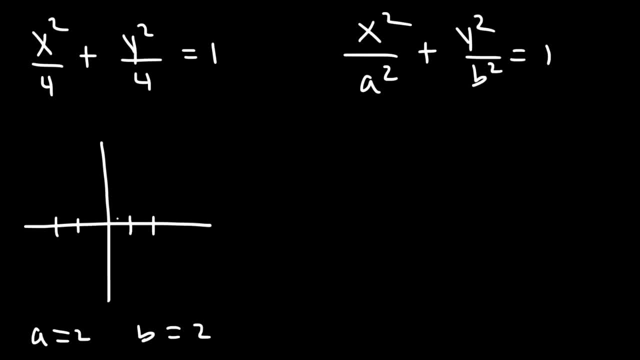 So is 2 and B is 2. So we're going to plot two points, two to the right and two to the left, from the center. We're going to go up 2 and down 2. So what we have is 2 left, 1 right, 1 right. flag Itu, 0 vão llegó você. 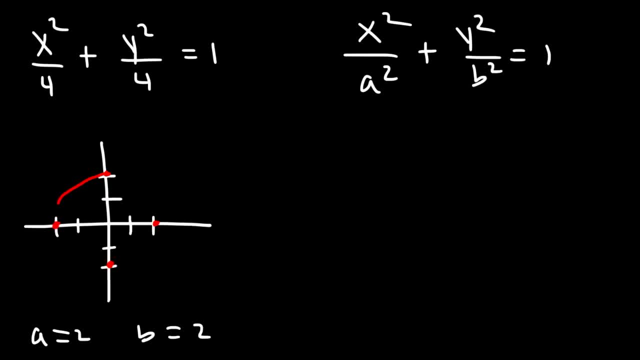 It's not an ellipse, but it's a circle, because a and b are the same. For an ellipse, c squared is equal to a squared minus b squared, so c is the square root of a squared minus b squared, and we know that a squared is 4, b squared is 4, so c is 0. C will always be 0 when dealing with a circle, and so the eccentricity is c over a, so it's going to be 0 over 2, which is 0. 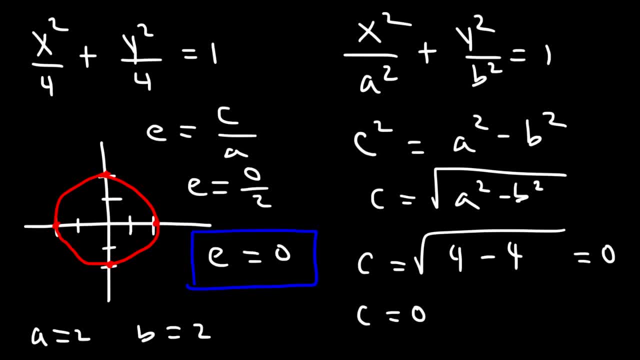 So whenever you have a circle, the eccentricity is 0, because a circle is perfectly even everywhere. 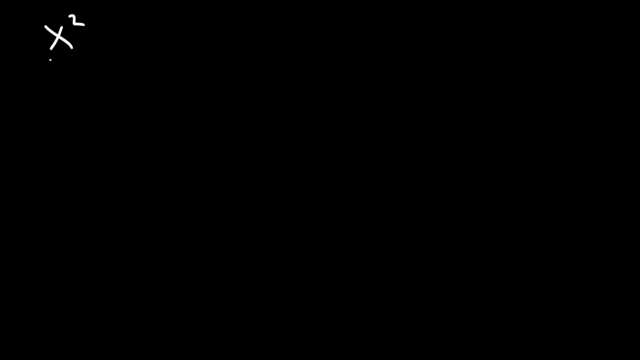 Now let's look at another example. Let's say if we have this equation, x squared over 9, plus y squared over 4. So because a and b are different, we have an ellipse. 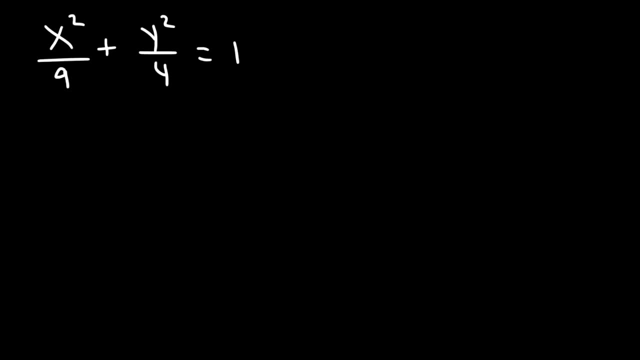 Go ahead and graph the ellipse, and calculate the eccentricity. So just like before. Okay. 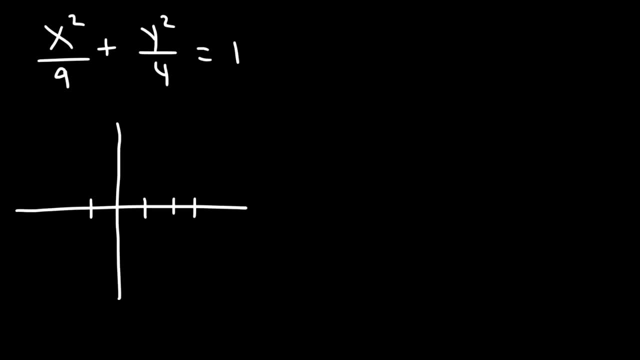 So this particular graph is centered at the origin. So a is 3, and b is 2. a squared is 9, so a is 3. b squared is 4, so b is 2. Now a is associated with the x variable, so we need to go 3 to the right, and 3 units to the left. 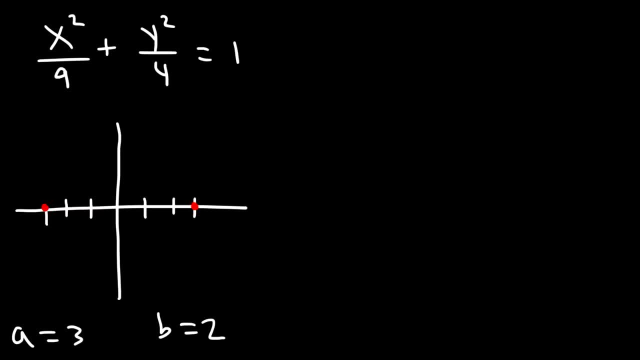 b is associated with the y variable, so starting from the center, we need to go up to y, and go up to units, and down to units. 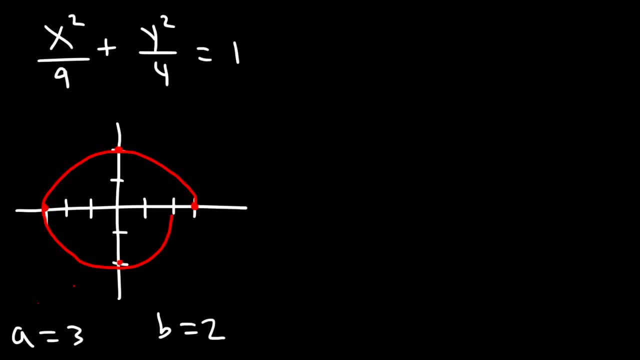 And then we can graph the ellipse. 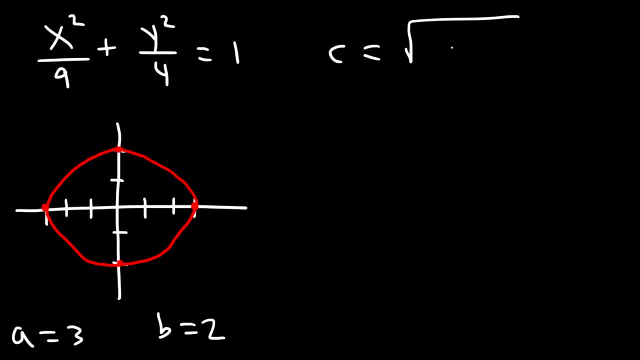 Now let's calculate the eccentricity. So c is going to be the square root of a squared minus b squared. And a squared is 9. b squared is 4. So c is equal to the square root of 5. The eccentricity will be c over a, so that's going to be the square root of 5, divided by a, which is 3. 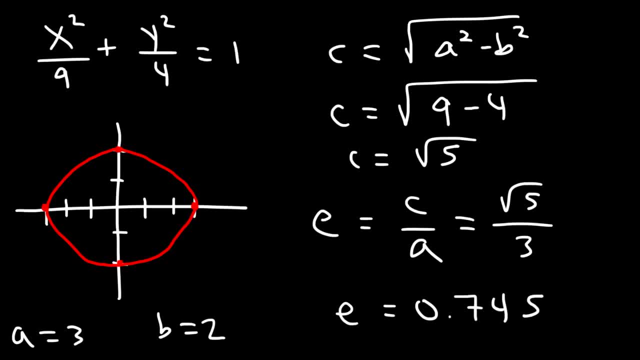 So that's 0.745. 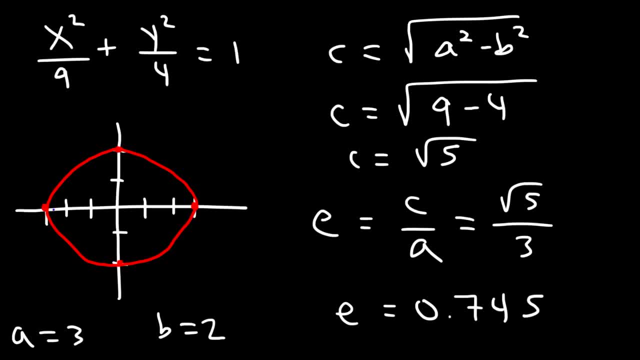 So as you can see, this ellipse is not circular. It's 6 units along the major axis. And the minor axis is 4 units long. 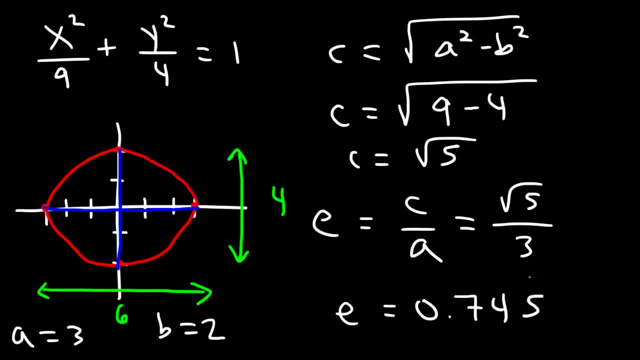 So it's a little elongated. And that's why e is significantly greater than 0. 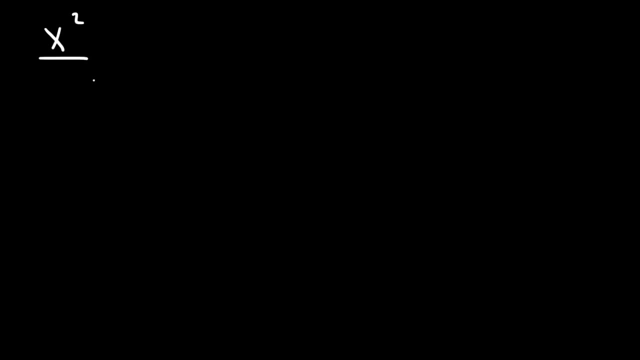 Now, let's consider one more example. So let's say we have the equation x squared over . Plus y squared over 1 is equal to 1.